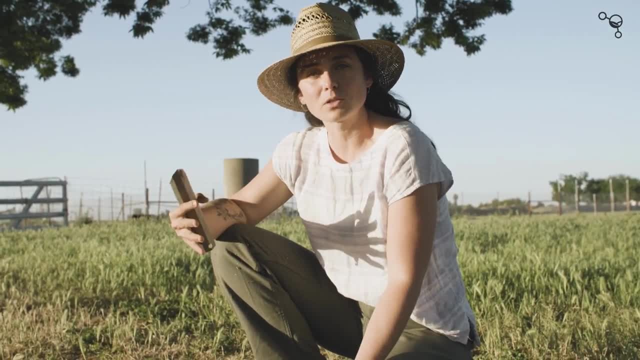 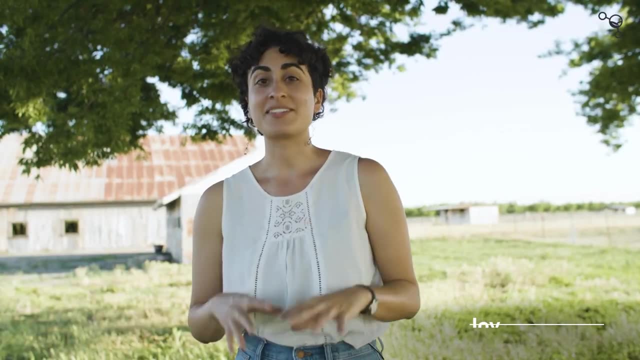 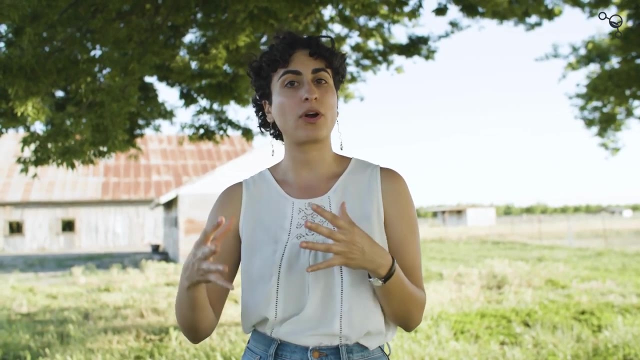 pathways to promote stress tolerance. We can bring in biostimulant or inoculant or some sort of carbon food for the biology. So now we're going to discuss a few different soil health management practices. You might be wondering: well, how do I get started? I want to learn more. 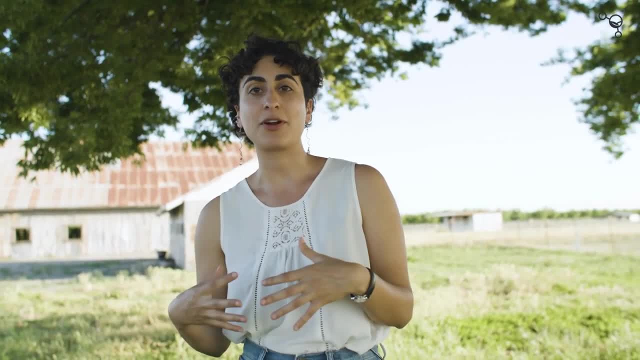 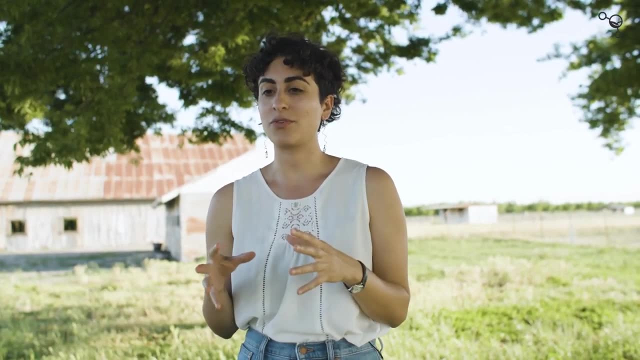 I want to learn about different ways to be regenerative on my farm or remediate my farm from where it's at today, Or you might be doing some of these and are interested in learning about more. So the first one I'll go over is cover cropping. Cover cropping is 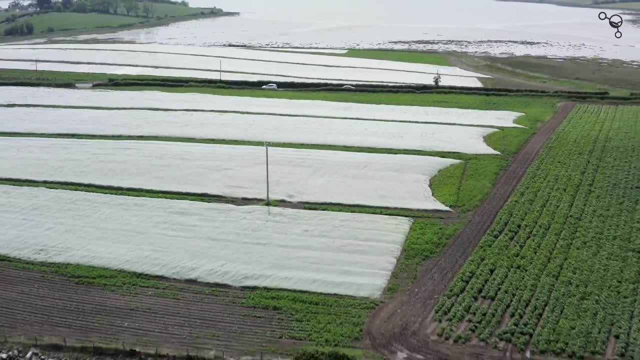 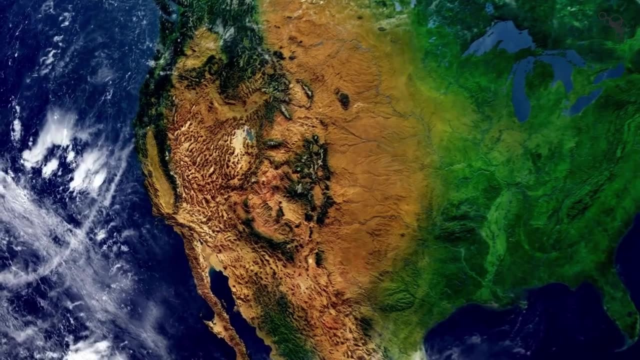 a great way to retain soil moisture in your field. It can also be used to fix nitrogen if you're planting leguminous cover crops. Cover cropping is not one size fits all. It really depends on your region and your soil type, So it's best to do some research on. 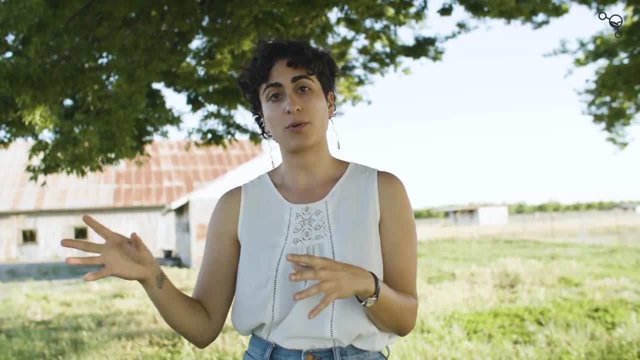 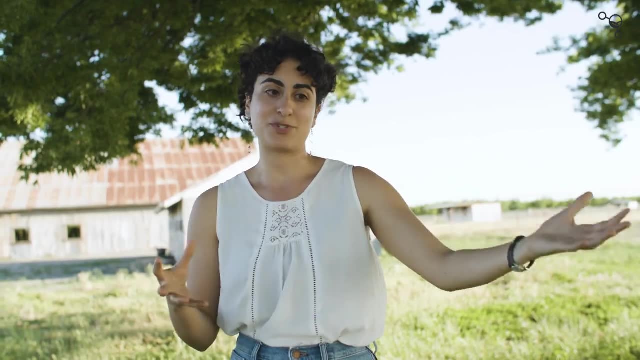 what will best serve your area And especially think about what you're going to be using and what crop you'll be growing after. But it's a great way to retain soil moisture and prepare for the next season, Because once you've harvested, before you've extracted. 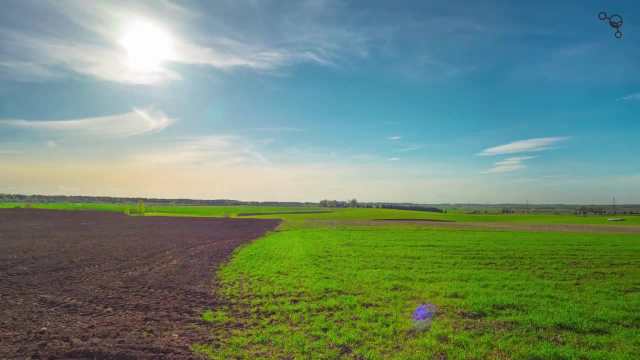 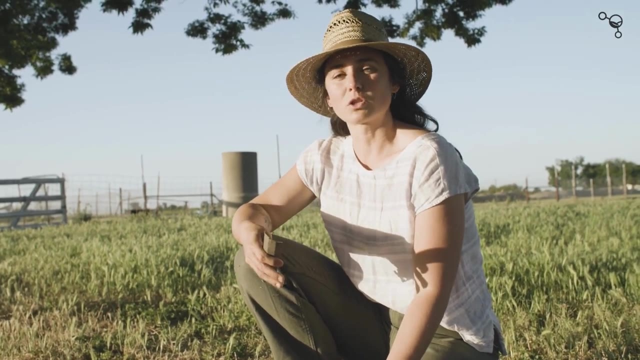 those nutrients and it's a good way to maintain them, bring them back and can even prevent soil erosion. And then we can start to think about minimizing disturbance. There's a lot of disturbance events that happen in agriculture today and that influences the soil microbiology. It's 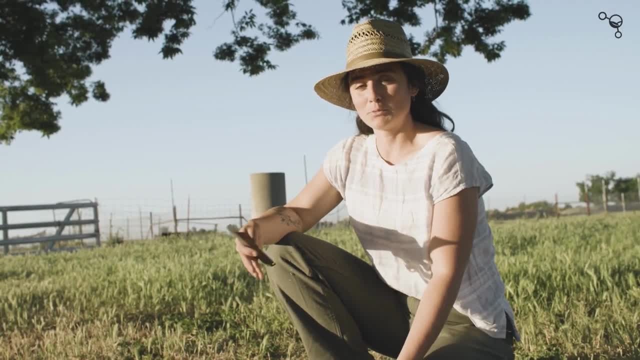 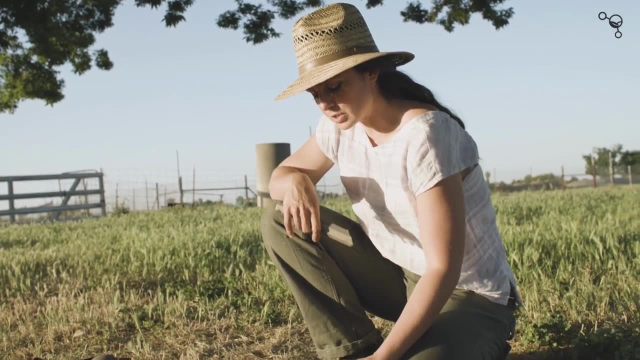 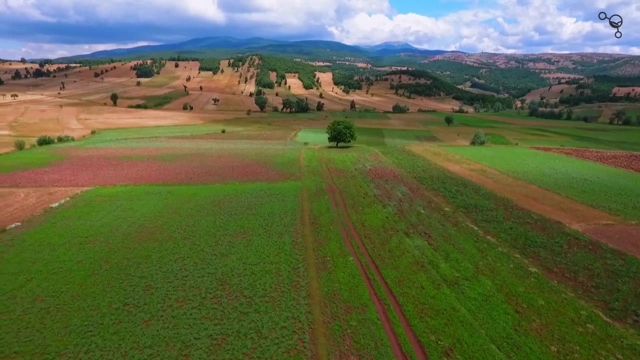 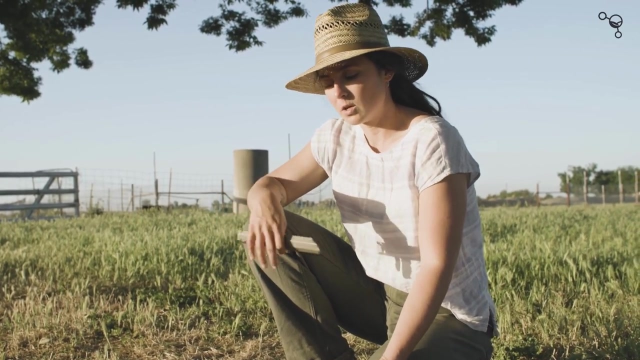 not good or bad. It's just we make observations scientifically That show us those. you know how that influences the biology So we can understand and consider how we're disturbing the soil and where we can reduce disturbance. And disturbance events can be. it can be both chemical and they can be physical. So tillage events are disturbance. 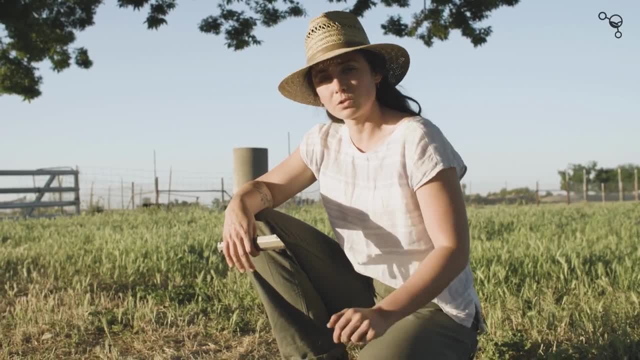 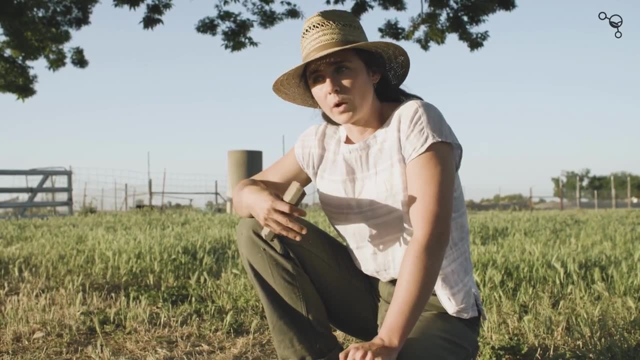 Where can we minimize tillage events? And then there's chemical disturbance too. So every time we use a fungicide, herbicide, pesticide, it disturbs the soil microbiology. So where in our management practices can we use other tools or limit some of those? 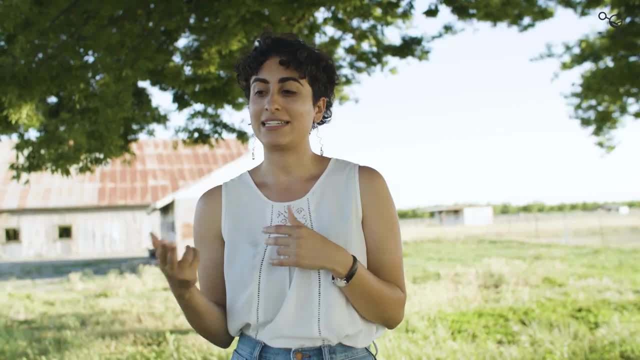 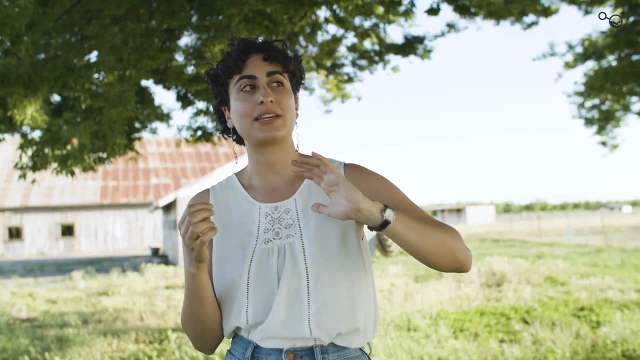 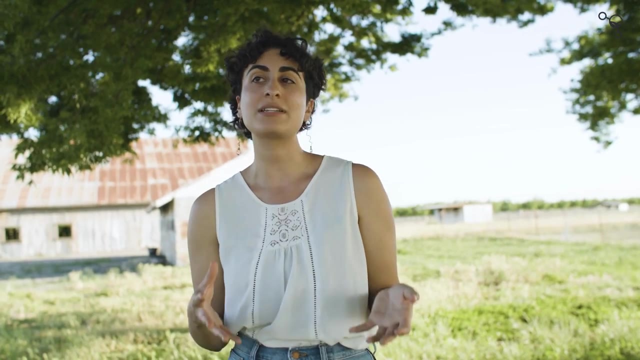 tools to minimize disturbance. Next, we can talk about livestock a little bit. There's rotational grazing, which is a great way to keep ground cover move animals around. There are lots of studies that show that rotational grazing can increase soil organic carbon, which is really important. 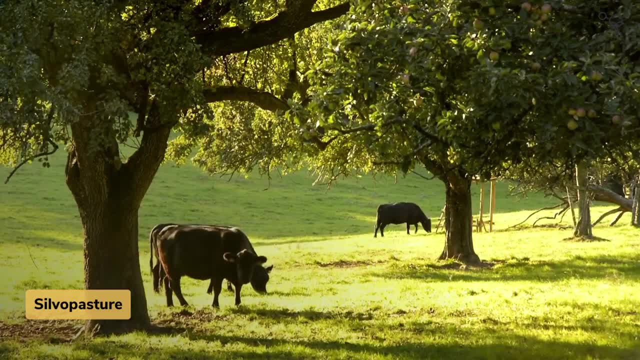 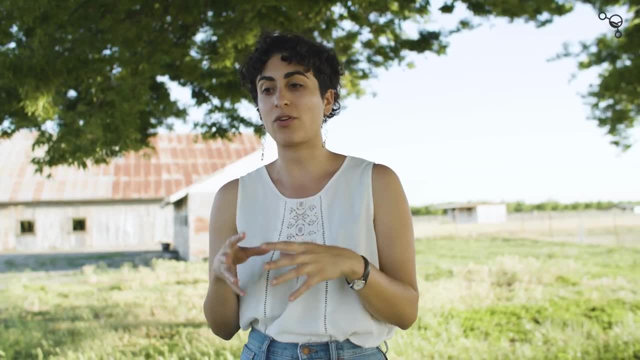 There's also silvopasture, where you integrate livestock with your cropping systems, So it's very hard to get soil organic. So it's really hard to get soil organic, So it's very harmonious. And lastly, there's intercropping, where you can be growing crops. Let's say 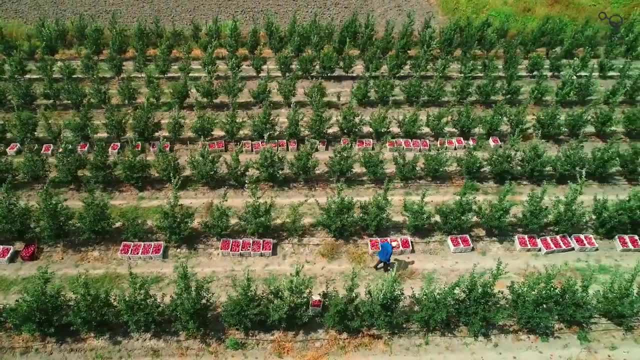 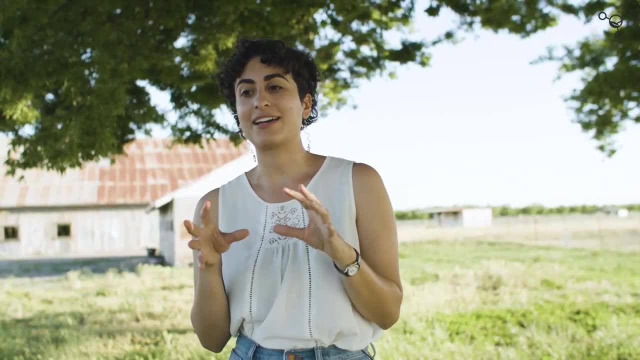 you have a vineyard or an orchard, you can be growing crops in the alleys to have ground cover, retain soil moisture, and it can even be a cash crop, So you're diversifying your farming plan. So then, talking about soil organic matter, another soil health management practice is: 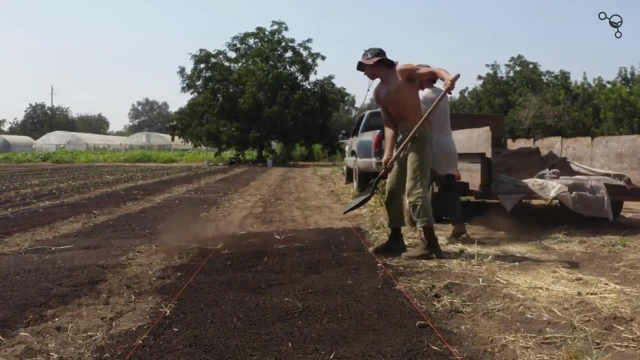 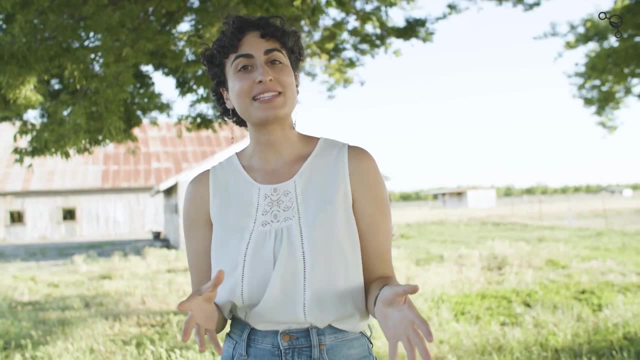 composting, So thinking about your farm. if you have livestock, recycling your outputs, using them as inputs, Applying compost is a great way to release soil organic matter, Depending on the frequency that you apply the compost at. that's something that we monitor. 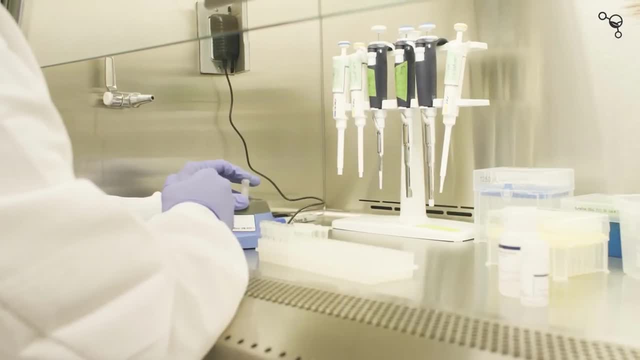 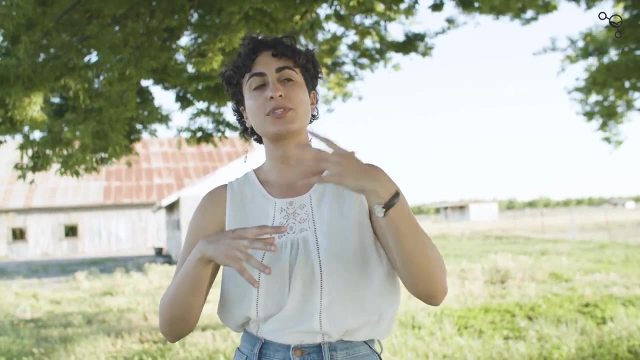 at Biome Makers, We can design trial tests where we're looking at the frequency that we're applying, the quantity we're applying. The last soil health management practice that I'll go over is biological products. If you are using chemical fertilizers and herbicides. 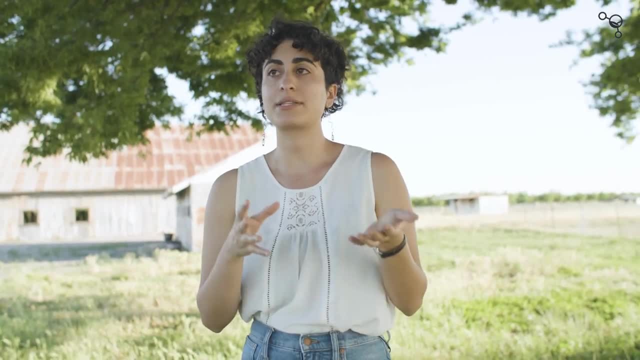 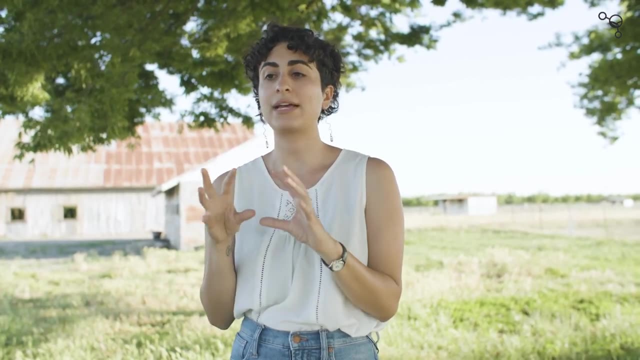 you're not getting the results that you want or you're just trying to move away from these products. One move is looking at biological products, biological stimulants, so you can think about the crop that you're growing, or the crop that you want to be growing, and look. 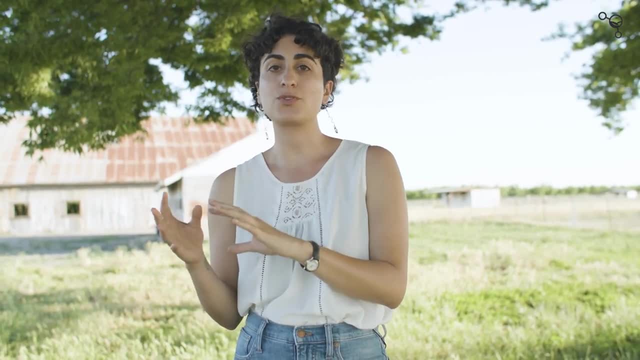 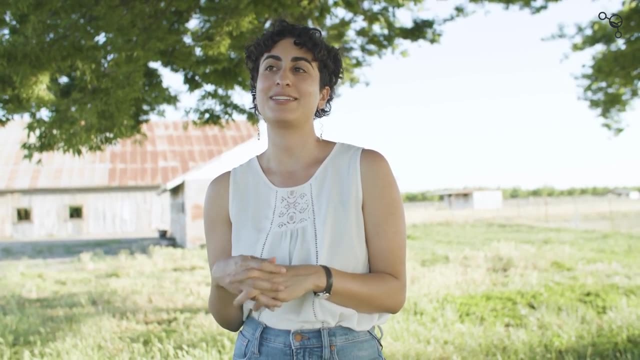 for a product that's good for the environment. So composting is a great way to look at soil that has the needed microbes or other nutrients that aid in your crops growth. so those are a few different practices when we're talking about soil health management in the regenerative world. 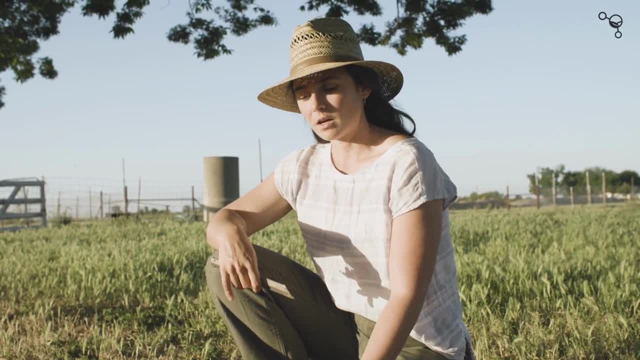 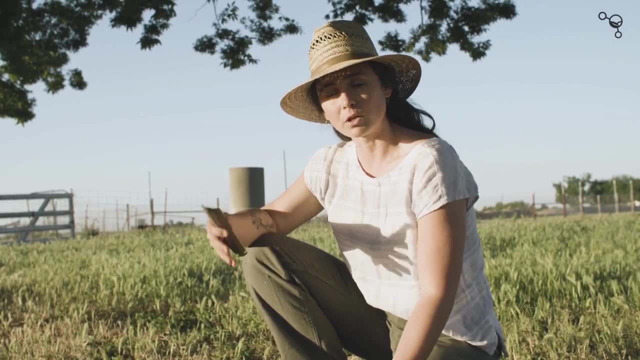 and then we can start thinking about the future and what we can do. next, we feed the biology- we've- we've recruited new biology- with biological inoculants like a compost tea or other manufactured products, and now we can think about what do we do in the fall? now, 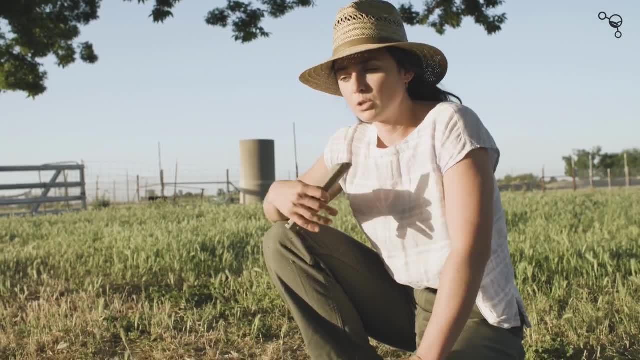 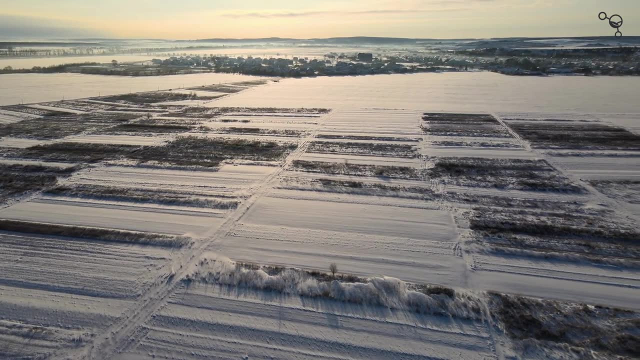 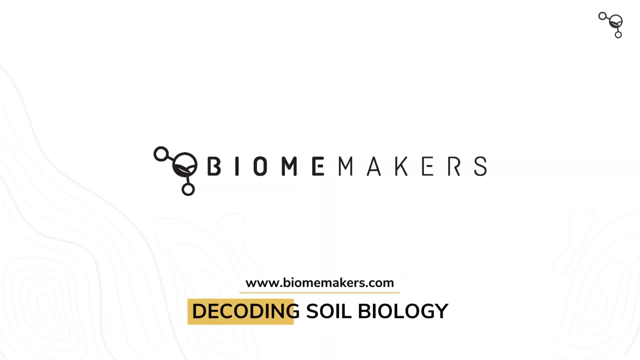 does a cover crop work work in our operation? can we do things to feed the biology after we harvest our cash crop throughout the winter, the off season, to replant into a healthier soil biology and ecosystem in in the next spring?